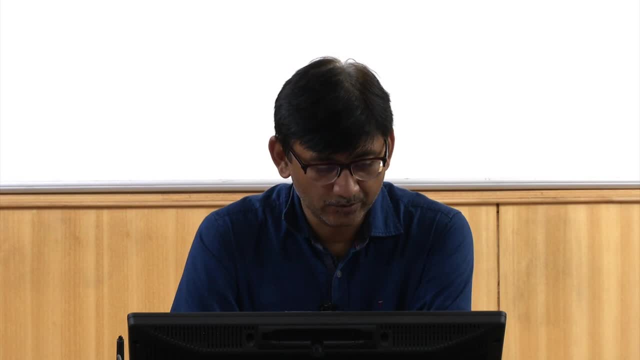 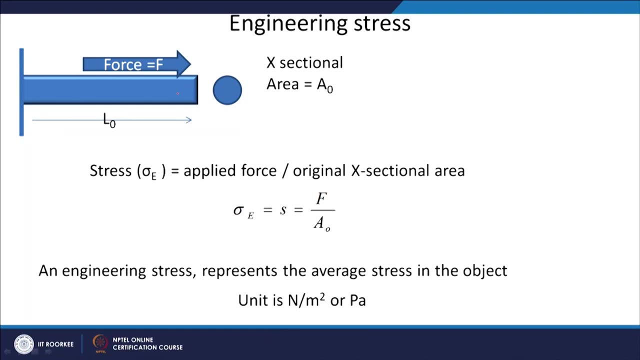 So first let us define the engineering stress. so basically this is cross sectional area. is there for a, for example, this sample and I am applying a force and it is kind of being at fixed at a particular point here and you are applying as force and this is the cross. 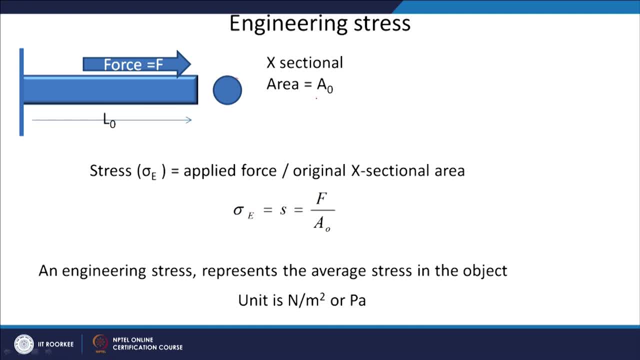 sectional area of this sample and that is given by A0 here, then the stress, which is the engineering stress here, which will be denoted by sigma E, is applied force divided by the original cross sectional area. So force can be applied or it can be the response of the material to the deformation. so if you 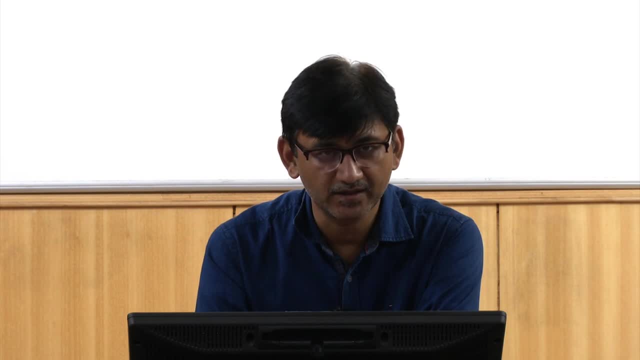 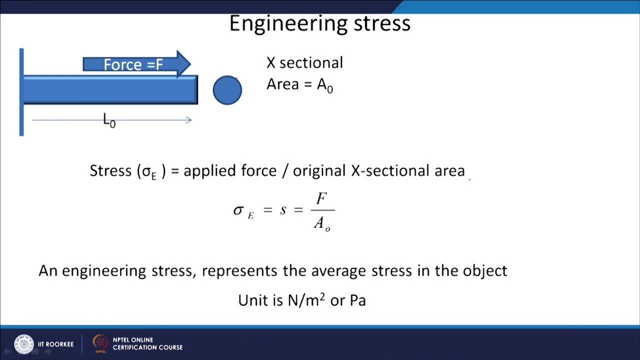 deform the material. The response of the material can be in form of resisting force or resisting stress. so that is, force divided by the original cross sectional area will give you the engineering stress. So we are now very specific that which area we are talking about here that I am talking. 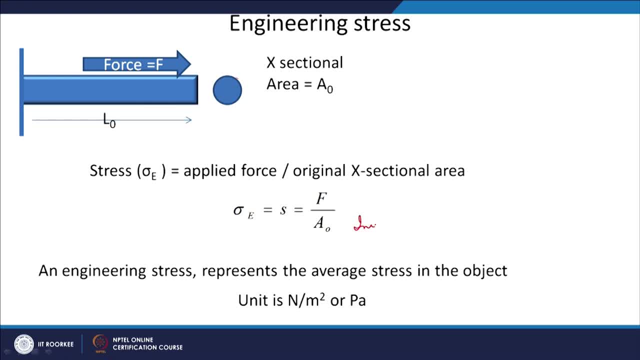 about the original or initial. So when we started the experiment, Whatever, What was the original cross sectional or initial cross sectional area of the material? we are talking about only that area divided by force. so force is divided by that area. of course, already we have talked about the units here. 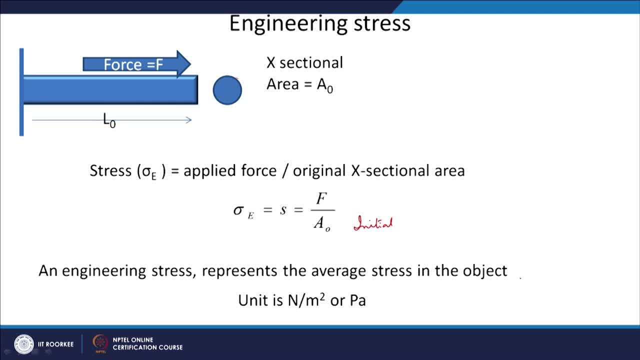 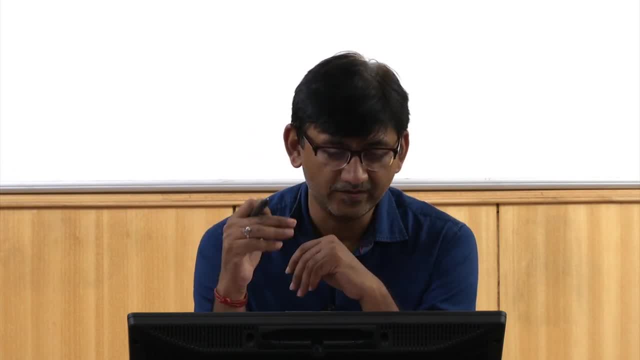 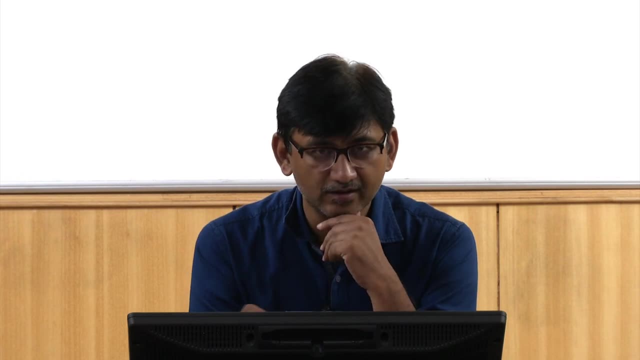 So an engineering stress represent the average stress in the object. so whatever is the average cross sectional area divided by the force is divided by this cross sectional area will give you the engineering stress, Engineering strain, if you want to define. so when we are again trying to deform the material, 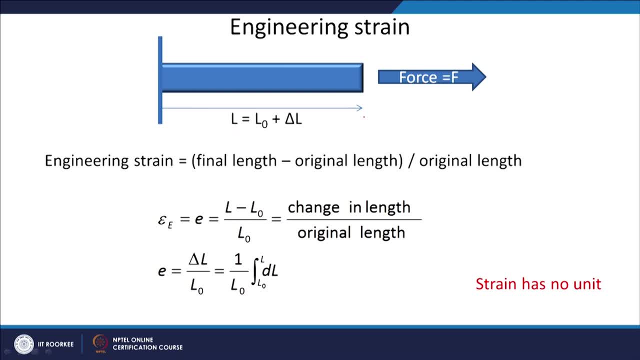 ok, So your now length, L is, will be equal to the initial length, L0, and whatever is the elongation or deformation which is delta L. ok, So initial length will be L0. that is my initial length, which has become L0.. Ok. 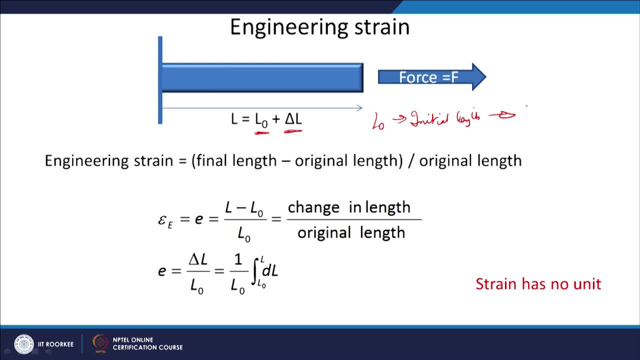 Ok, Ok. So this will become L after deformation. So after deformation this has become L. So L is equal to L0 plus whatever is the deformation delta, L. So any engineering strain, if I want to know that, will be equal to final length. 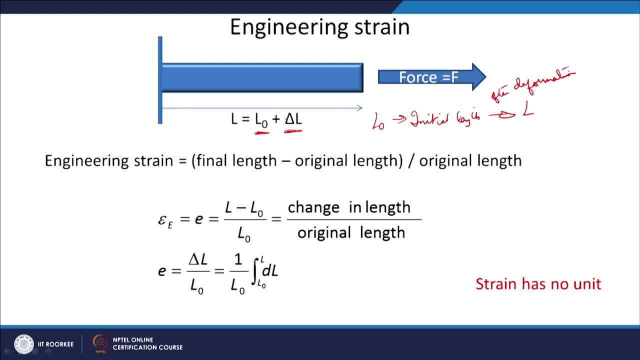 minus original length divided by original length. ok, So basically delta L. Already we have seen, We have seen the delta L divided by L0.. So delta L contains the final length, L minus L0. ok, that is my going to be my delta L divided. 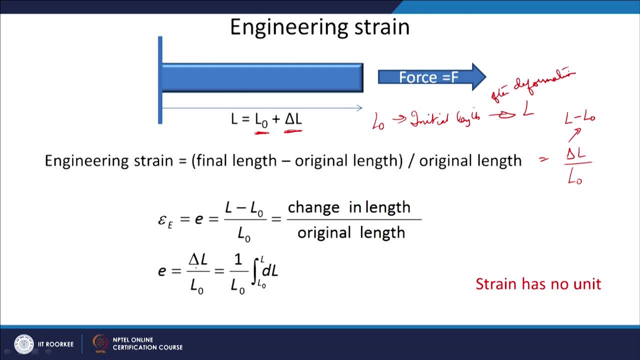 by original length. So in some mathematical terms I can write it as epsilon e sub e, or I can just say that with a small e, which I am saying that it is engineering strain, It is engineering strain that will be equal to L minus L0 upon L0. 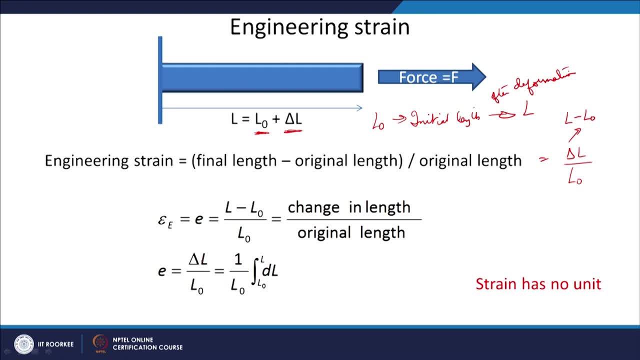 So that is change in length upon original length. ok. So delta L upon L0, as I told you, ok. or in terms of: if you want to integrate over all the deformations, ok, then it will be 1 by L0, integration from L0 to L into DL. 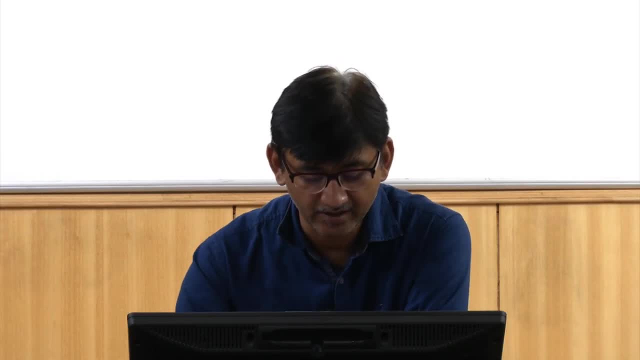 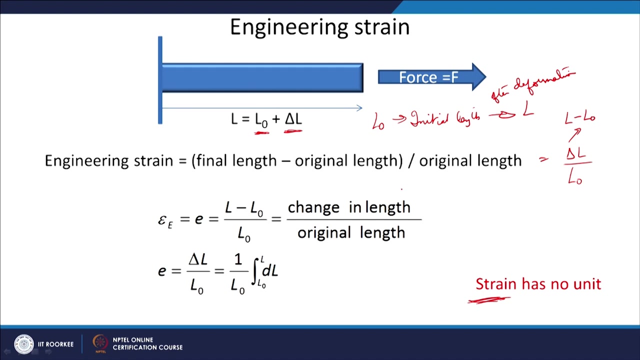 So suppose if I am doing the deformation in increments, I can just do an integration like this to get the total strain in the engineering, strain in the material. ok, Important thing to notice: that strain has no unit. ok, Because we are dividing by length, by length, so there is not going to be any unit for strain. 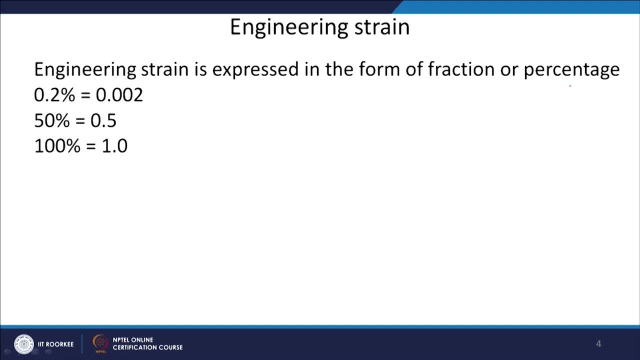 Engineering. strain also is expressed in form of fraction or percentage. ok, So either we will say be saying 0.2 percent. ok, If you remember, this is what we said when we were trying to find out the yield strength of a material. Ok, 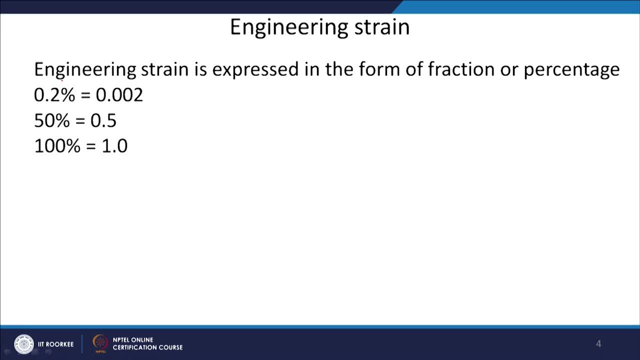 a stress-strain curve, which is a continuous stress-strain curve. So we found out the yield strain after a 0.2% of permanent strain or plastic strain. In fraction it will be 0.002,. 50% will be equal to 0.5,, 100% will be equal to 1,. okay, 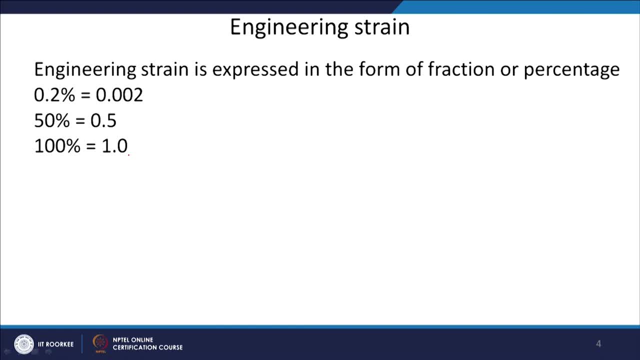 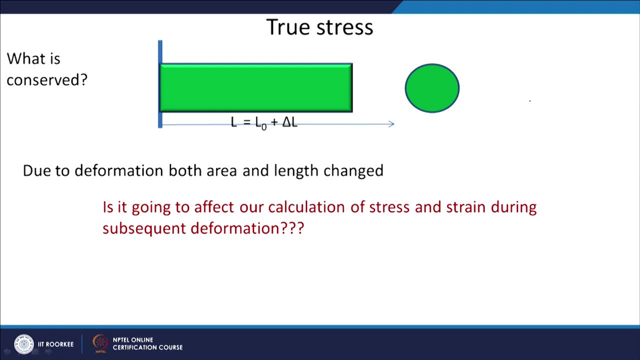 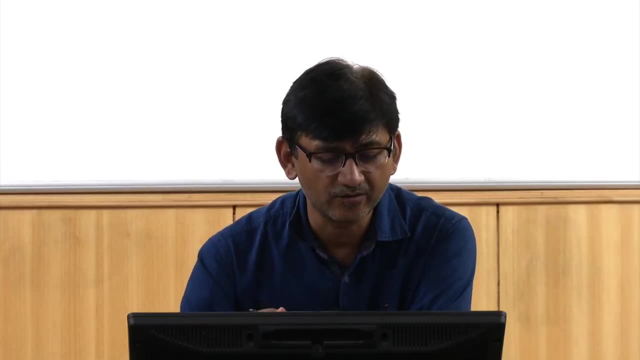 So you can express it in different forms: fractional forms or in percentage. Now the question is that when I am deforming a material, okay, initially, when you are in elastic part, the deformation is very small and you will not be able to notice that. okay. 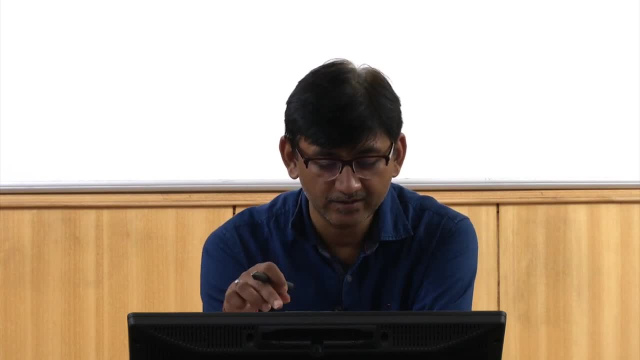 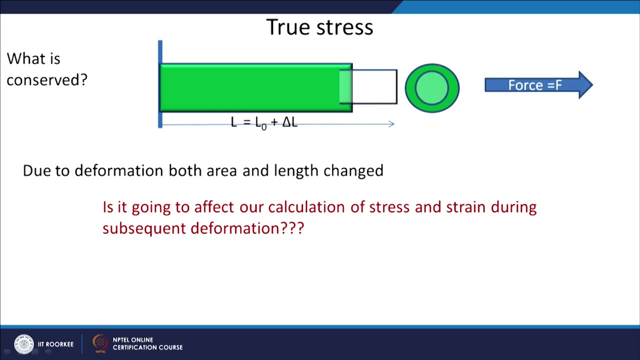 But if I am going into plastic deformation, what will happen? This is my some bar with this cross-sectional area. okay, I am applying a force. okay, and after some deformation, Now the cross-sectional area has reduced. okay, and the length has increased. okay. 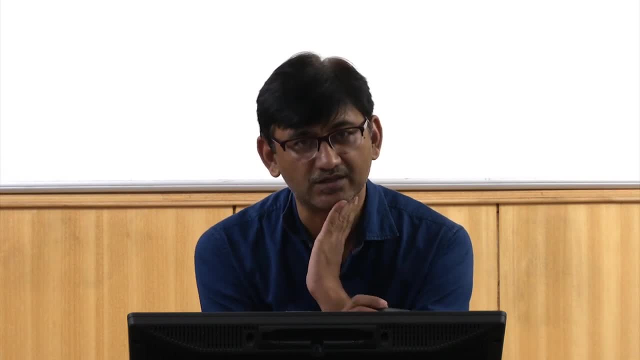 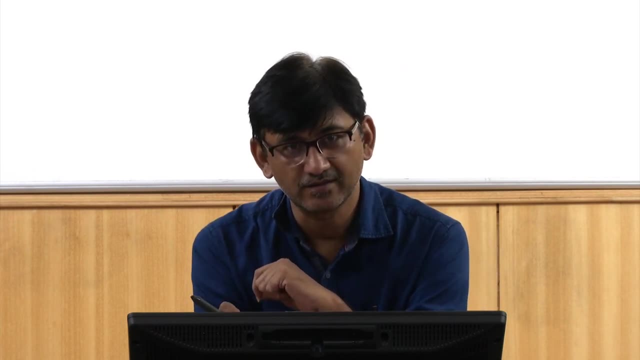 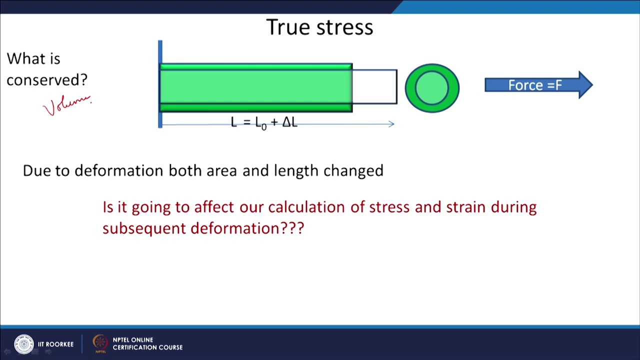 So a question is posed here: what is conserved here? okay, So what is conserved here is volume. So whatever is the increase in the length, the decrease in the cross-sectional area will be proportional, and that will be can be found out by volume, okay. 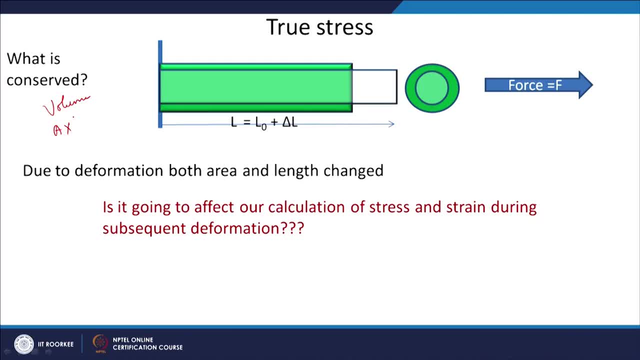 So my cross-sectional area is A, into, So initial length is L0,. okay, That will be equal to A, the final cross-sectional area and A final length. okay, So length will increase, So cross-sectional area has to reduce will decrease. 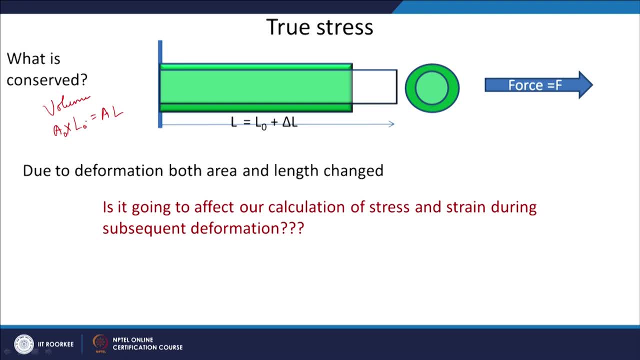 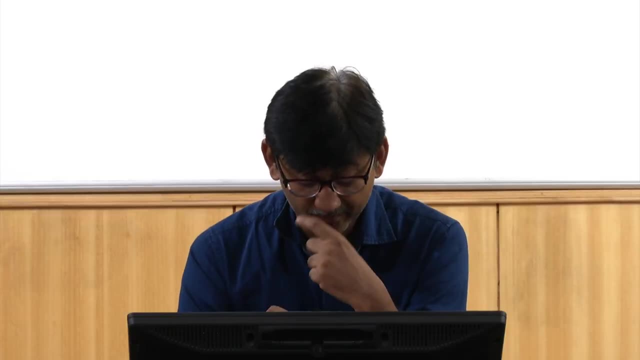 So that the overall volume constancy will be going to be there, So volume is going to be conserved, okay. So in this case, my length is increasing, My cross-sectional area is reducing, okay, Okay. Now the problem or the question which we want to pose here is that when I am finding out, 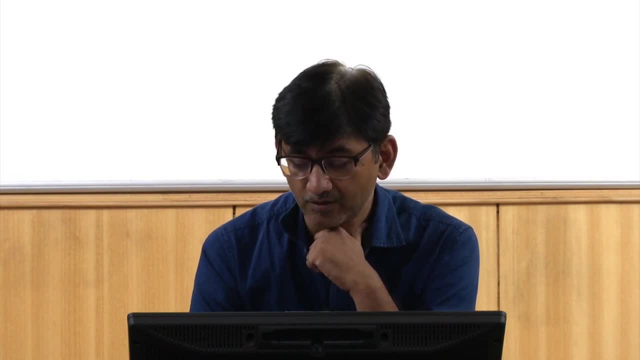 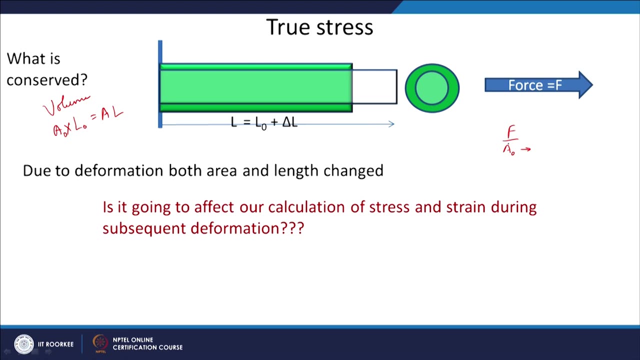 the engineering stress. I said the force divided by the original cross-sectional area A0. But now, during the deformation, my area A itself is changing okay. So you can see that area has reduced okay. So my cross-sectional area has come down okay. 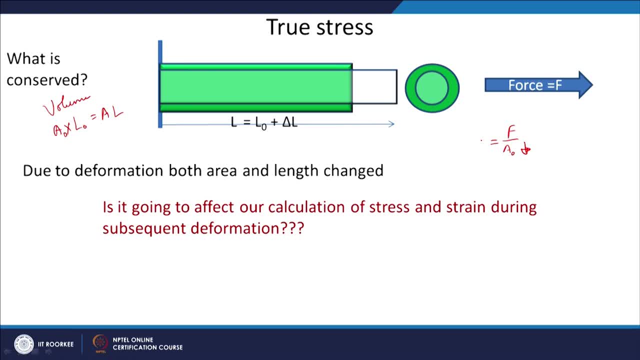 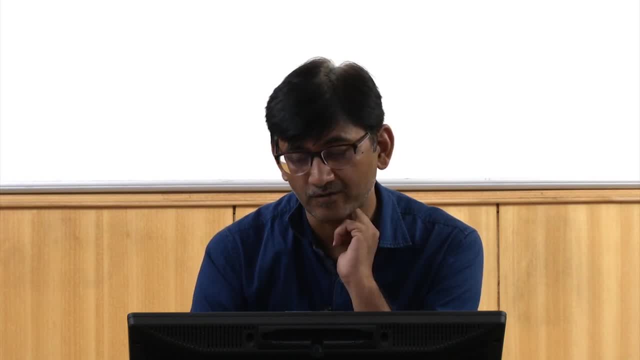 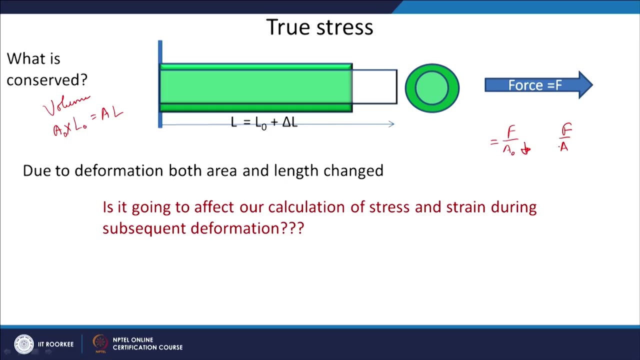 So the stress which we are calculating from engineering stress, Okay, The stress relationship. that is not correct. That is not the stress which the material is experiencing. okay, The material is experiencing the stress which is given by force divided by the instantaneous area. 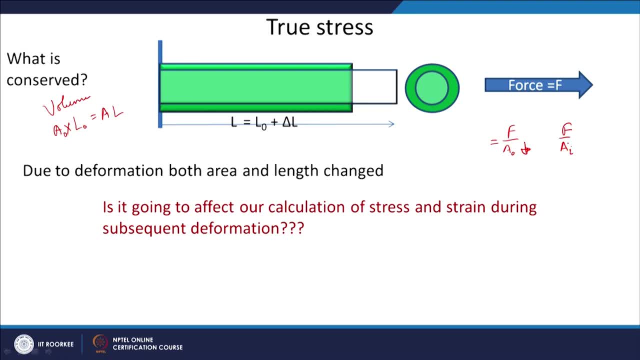 Let us say I call it as Ai, okay, So, because my both area and length are changing, it is. is it going to affect our calculation of stress and strain during subsequent deformation? So that is what I am trying to answer here. That is what I am trying to answer here. 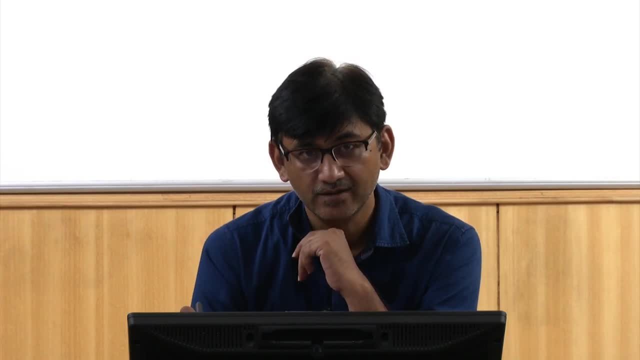 Because my cross-sectional area is reducing. okay, the stress calculation which I am doing from engineering stress expression is not going to be the actual stress with which the material is experiencing. okay, What material is experiencing is because of the cross-sectional area Ai, which is now force. 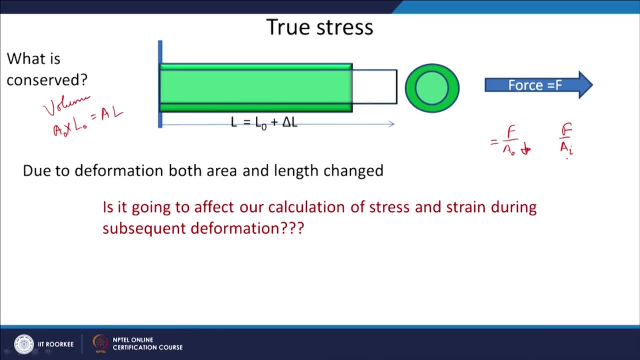 divided by Ai. okay, So that is what we call as true stress. So true stress is when I am dividing the force by the instantaneous area. So that is what we call as true stress. So true stress is when I am dividing the force by the instantaneous area. 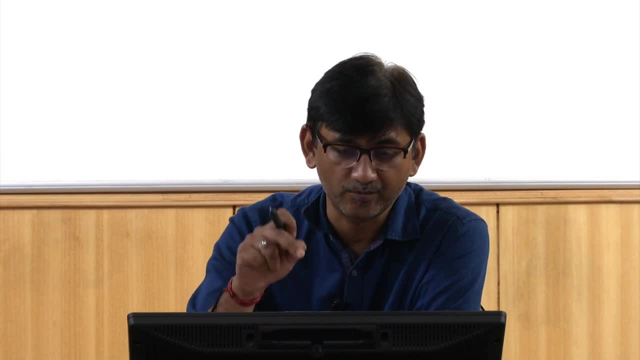 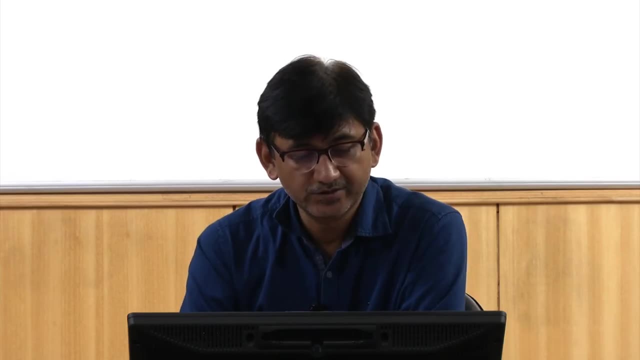 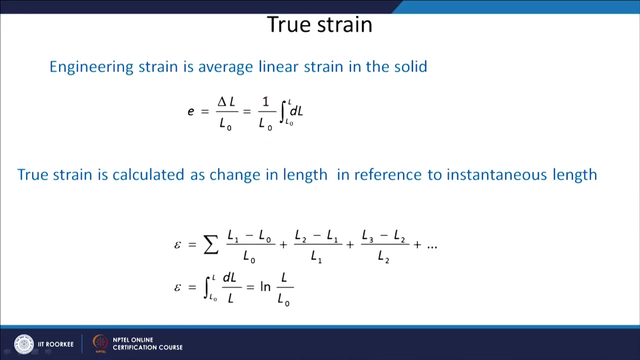 Okay. So true, stress can be defined as load divided by instantaneous area. So, true, stress can be defined as load divided by instantaneous area. Similarly, true strain. okay, because length is going to change. okay. So engineering strain, we defined as a delta L by L0, which was written in integration form. 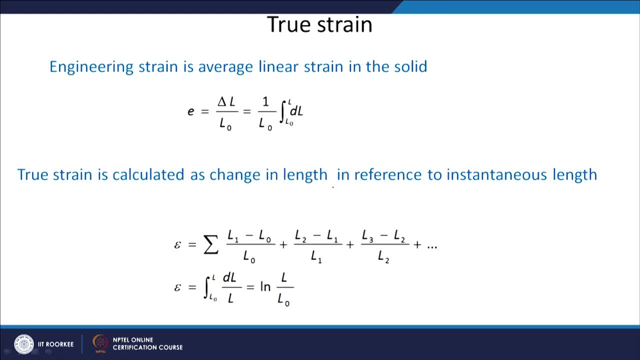 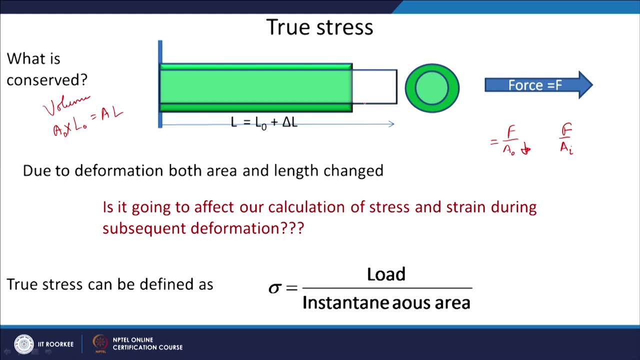 like this: The true strain is calculated as a change in length in reference to instantaneous length. okay, So whatever we discussed in case of stress, that will be dominated. Okay, Babaji, alright, be true in case of strain also. so, for example, for the first case right now, the change in 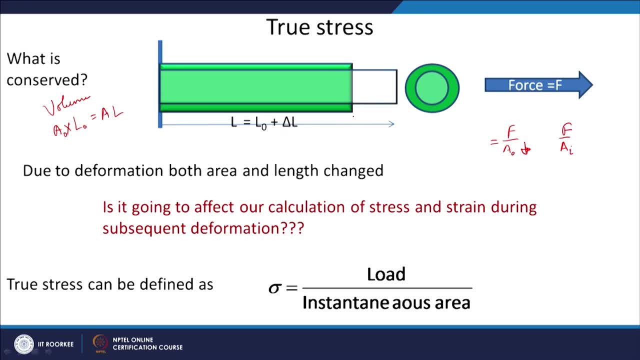 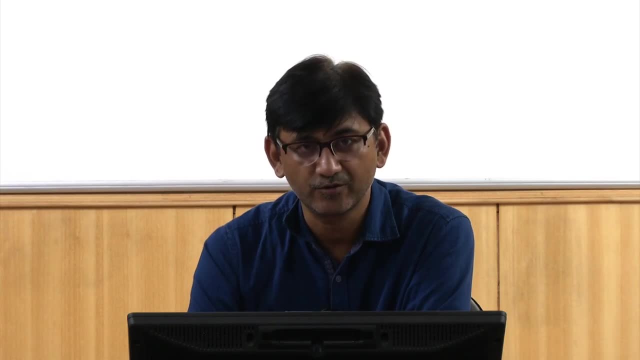 length is delta L divided by the L0. that is my, going to be my engineering strain now, for subsequent deformation when the length is again increasing to some other value. if I divide it again by the initial length, the strain which I am going to get is not the correct strain, because in between my length has increased to L. so for subsequent deformation I should use the actual length of the material to get the strain. and that is what is the problem. So now for true strain. what we will do, we will do. we will also take the instantaneous. 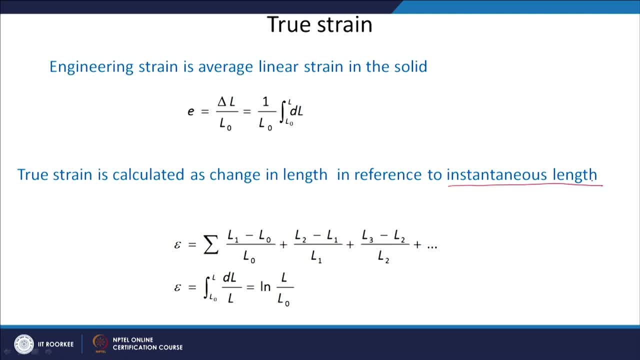 length rather than the original length. so now the summation. if you want to look so, it will be L1 minus L0, so there will be like: initially the length is L0 and in subsequent deformation it is becoming L1, L2, L3, so what? we are saying that for each of these, 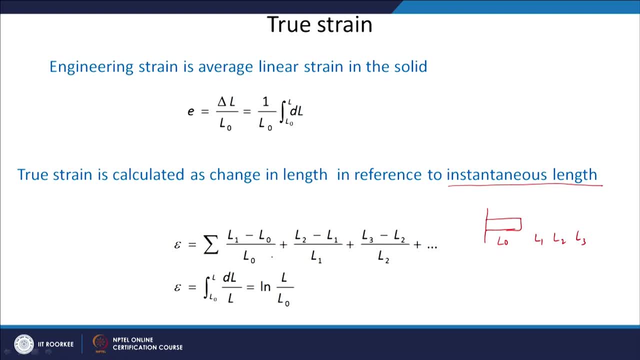 increments. so it will be L1 minus L0 divided by L0, then L2 minus L1 divided by L1, then L3 minus L2 divided by L2. that should be the true strain If you compare this with the engineering strain, in that the summation will be like this: L1. 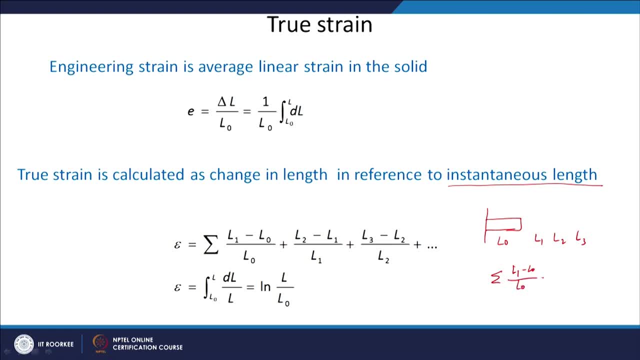 minus L0, divided by L0 plus L1 minus L2 minus, it will be L2 minus L1 upon L0, plus L3 minus L2 upon L0, and so on. so in all case you will have in the denominator you will have L0. that 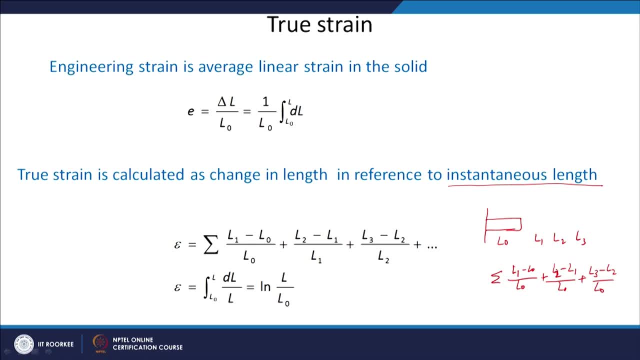 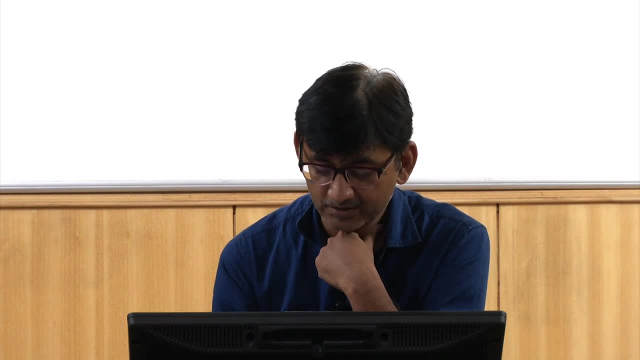 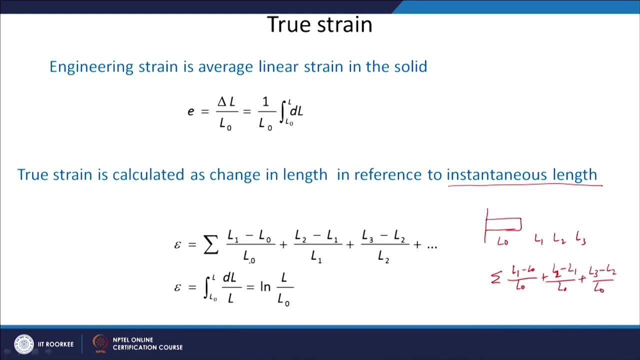 is what we have taken out And basically you are doing summation over here. so that is what is the integration we are using in DL. so if I took this type of summation for true strain, what will happen? my length is now continuously changing. so first increment, it was L0, second increment: 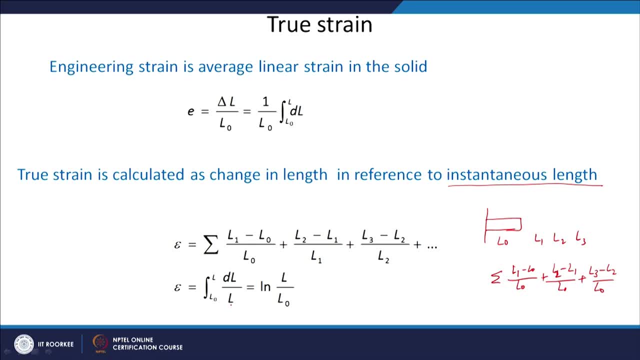 L1, L2 and so on. so it will be now DL by L and the integration is lower limit, L0 to L. So integration of this type will give you quantity in terms of basically, so integration here will give you L0 to L. so if I put it, it will become ln L minus ln L0 and in logarithmic, 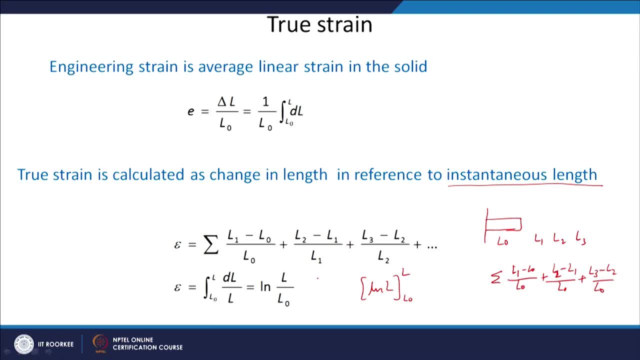 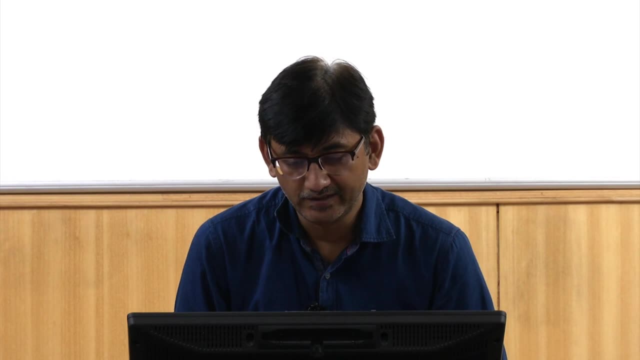 terms, it will become ln, L upon L0.. So this is what you will get in case of true strain. That is why we call this strain as logarithmic strain also. now, what is the advantage of true strain calculation? that is very important, so let us do engineering strain calculation. 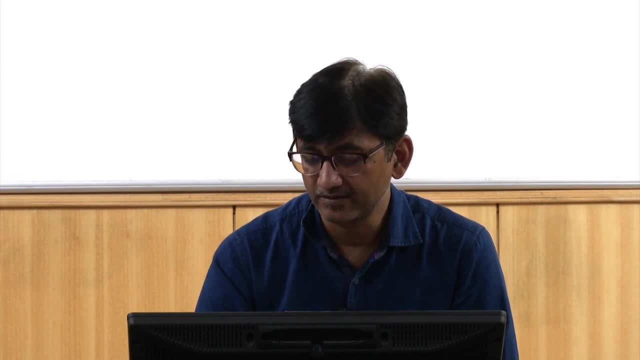 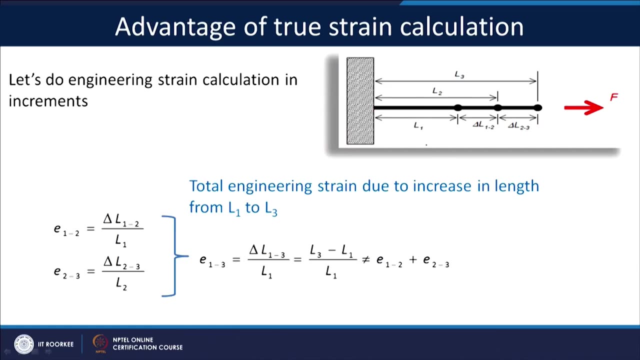 in increment. so your initial length is L1, then it increased to L2 after first increment, then it increased to L3 after the third, second increment, and so on. So this is from 1 to 2, it is delta L12, from 2 to 3 it is delta L23, and so on. so engineering. 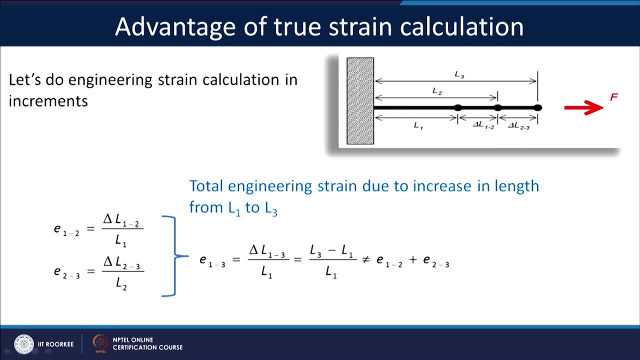 strain. if I want to calculate between 1 and 2, it will be delta L12 divided by L1, E23 will be equal to delta L23 divided by L2, and so on. And if I want to do the whole deformation in one go, for example, rather than doing in, 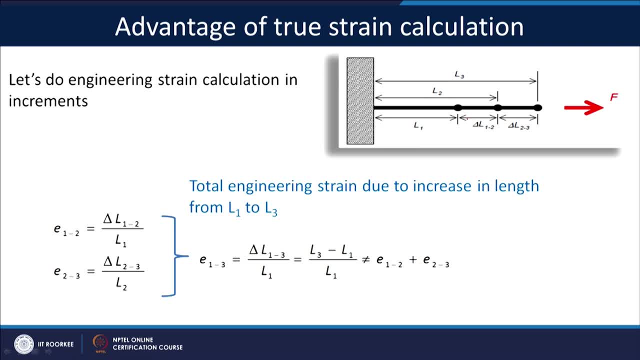 this increment. Suppose I want to take this particular deformation from directly from L1, the initial length, to the final length, L3, then I will say that the strain is equal to E13 delta L13 divided by L1, which will be equal to L3 minus L1 upon L1.. 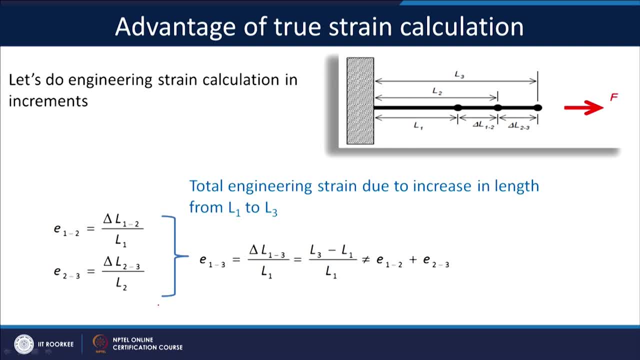 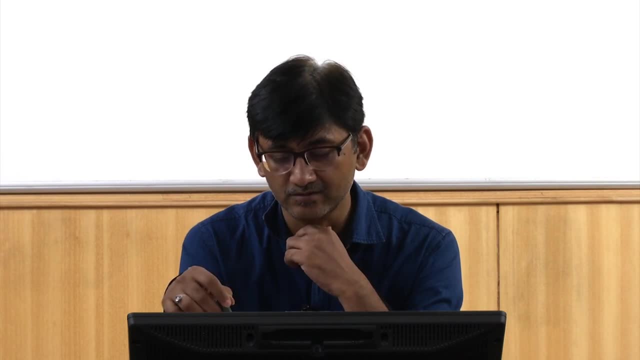 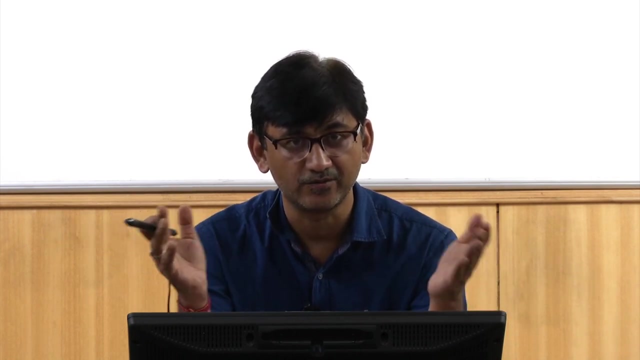 Now the thing which we want to compare here, whether this two increments are equal to this one single increment. Okay, See. So dimension, in both the cases, dimension of the my material is going to same, going to be same. So L1 to L3, so that is one quantity which is there, which cannot be changed. 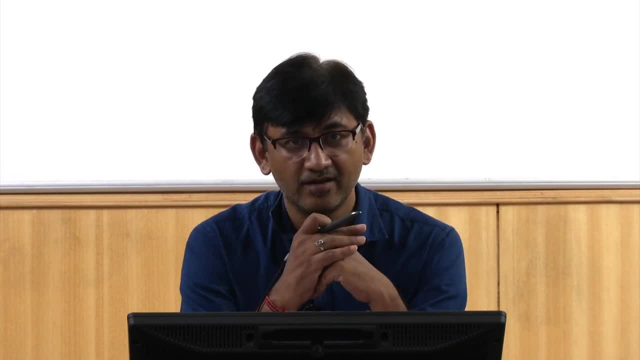 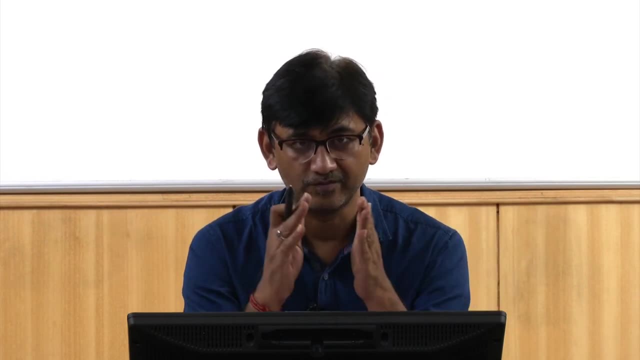 You know that length has increased from L1 to L3.. In one case we have done this in increments. in second case we have done it in one go from one, from L1 to L3.. But if you compare, if you do a summation here, 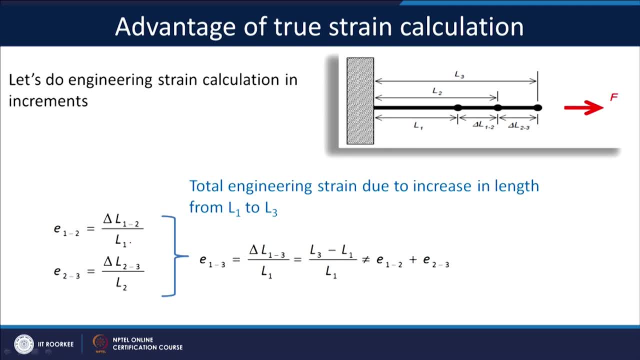 Okay, Then the summation of these two. Okay, You can do a summation very simple. Okay, You, L2 will be multiplied here, L1 will be multiplied here. Okay, And bottom, you will have L1, L2 and so on. 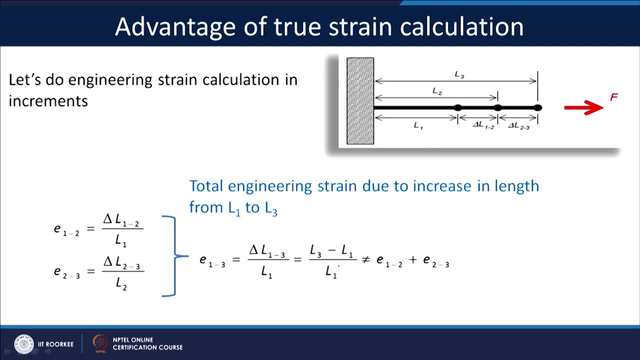 Now that quantity is not equal to this, Okay, Is not equal to L3 upon minus L1 upon L1, or in terms of delta L, if you want to write. it will not be equal to delta L13 upon L3.. Okay, So when we are taking engineering strain, 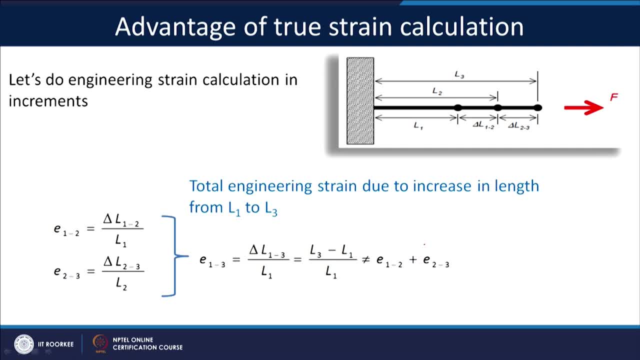 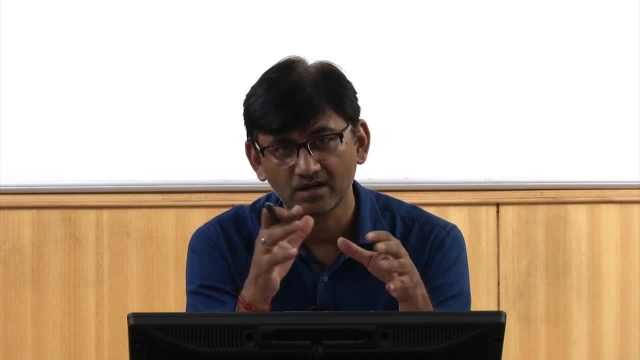 Okay In increments, and if you go in one shot, the strain in both the cases, the calculation of strain in both the cases or the value of strain in both the cases is not going to be same. So that means there is some problem in engineering calculation of engineering strain. 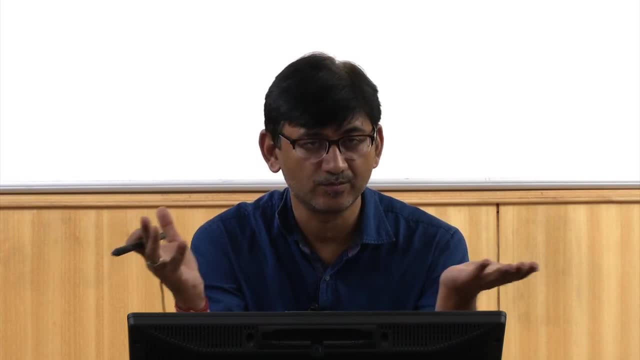 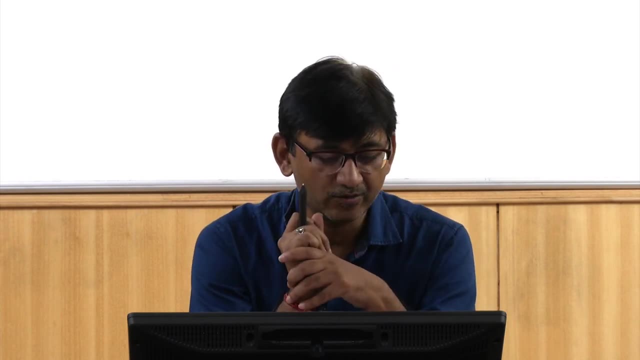 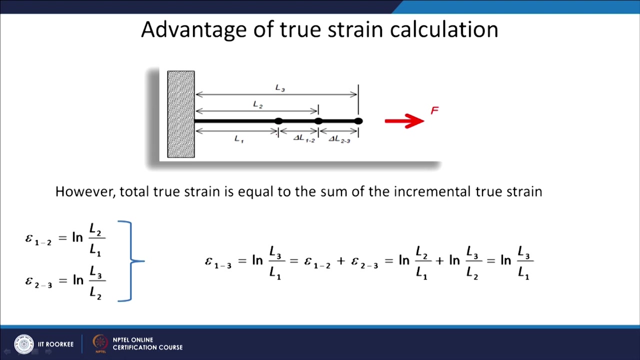 Because if my length is going to be same, the engineering, in both the cases, strain, should come same. Okay, And that is where the importance of true strain calculation comes. Okay, Now let us see do the same calculation with true strain. Again, we are doing first case in increment L1, then from L1 to L2, from L2 to L3.. 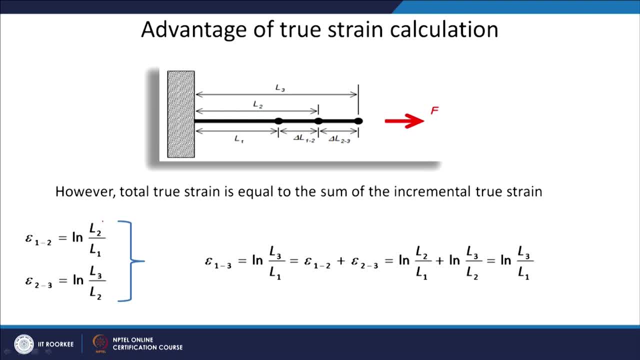 Okay. With that is written here: epsilon 12, so it will be log L2 by L1, epsilon 23, log L3 by L2.. Okay, And if I want to do in one shot, It will be epsilon 13.. 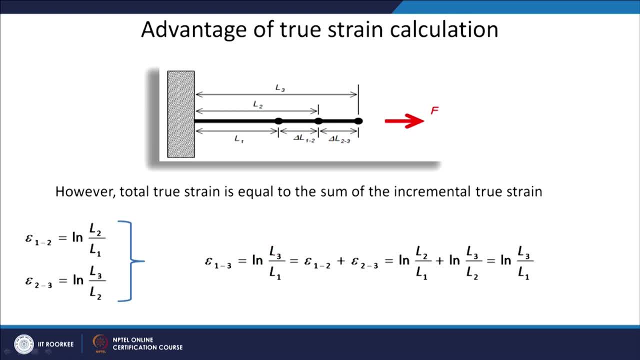 Okay, So epsilon 13 will be equal to log L3 by L1.. Okay, We are going directly from L1 to L3 and this: we are going from L1 to L2, from L2 to L3.. So, in increment, here we are going in one step. 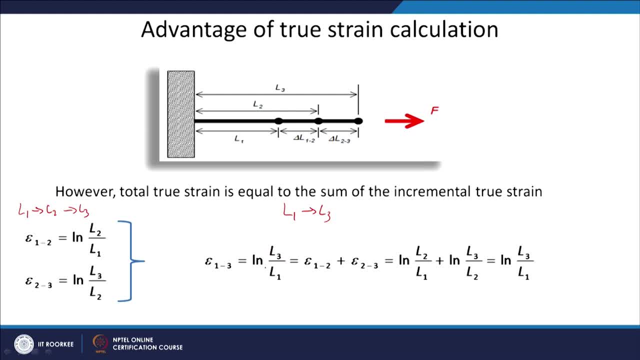 Now we have to see that, whether this is equal to this or not. So I am doing a summation here: epsilon 12 plus epsilon 23.. I am writing in logarithmic form: Log L2 by L1. this is plus log L3 by L2.. 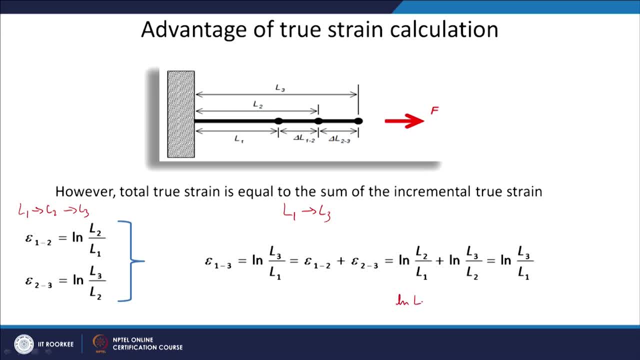 Okay, So if I expand this, it will be log L3- L2 minus log L1, plus ln of L3 minus ln of L2.. Okay, So, if you see this, I will cancel both. this is negative and this is positive. and now this: 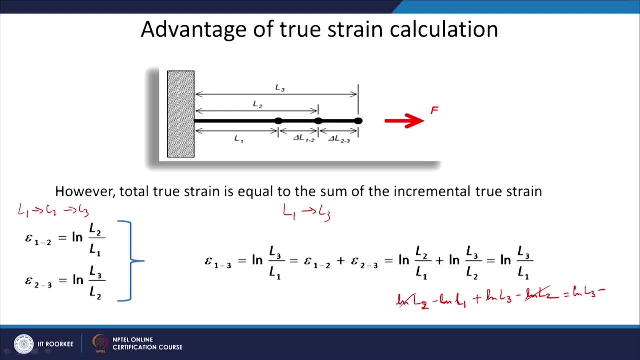 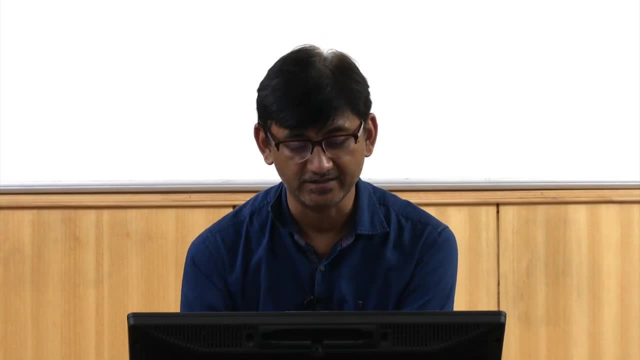 I can write as ln L3- L2.. So this is L3 minus ln L1.. Okay, What do you mean by ln L3 minus ln L1?? This is ln L3 upon L1, which is same as what we have got in the first, in one single step. 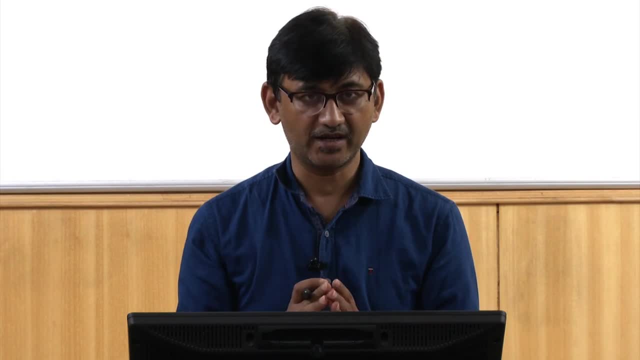 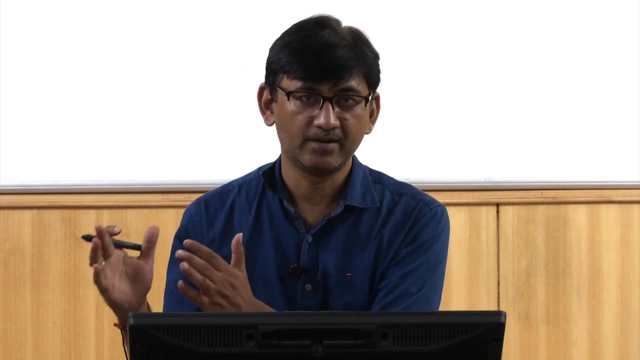 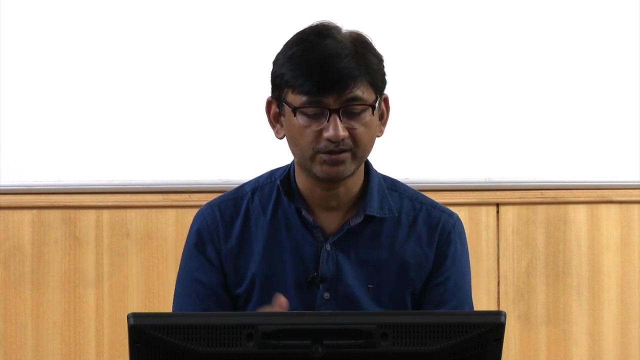 So with true strain, the importance of true strain calculation is that I can, if I do some strain in increments, Okay, And if I do the same deformation in one step, The amount of strain will be same if we do calculation using true strain, and that is. 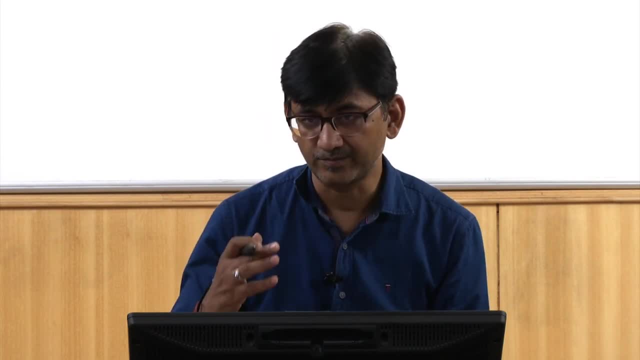 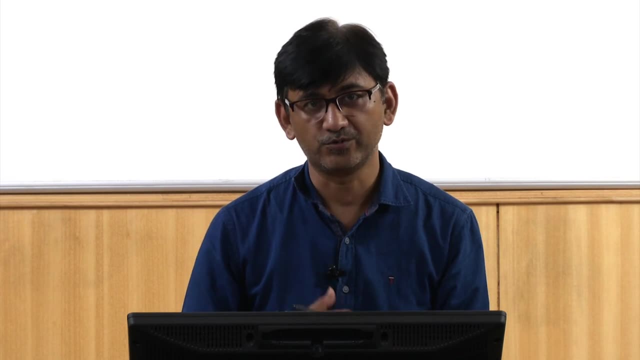 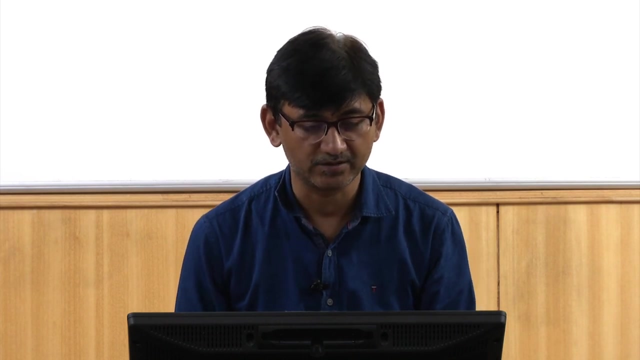 very important in material processing, where, sometime, deformation are done in stages. So the calculation of strain is going to be same whether you do in stages or if you do in one step. Okay, And that is why true strain calculations are used in all the material processing industries. Okay, We also relate the engineering stress or strain with the true stress and strain. Okay, So here we are finding out the relationship between engineering and true strain. Okay, So if I want to write engineering strain, it will be delta L by L0, the initial or original. 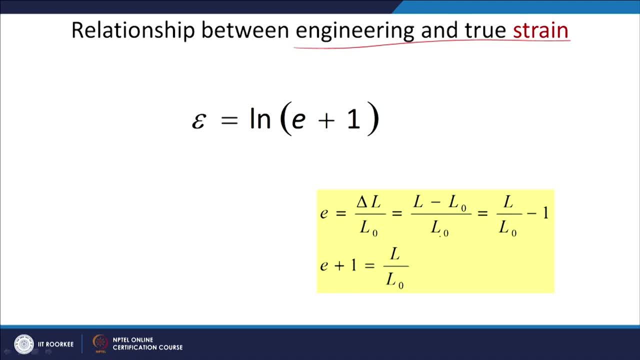 length, which I can write as L minus L0 upon L0.. Okay, L is your final length minus initial length divided by initial length, which I can write like L upon L0 minus 1.. Okay, So I take L upon L0 minus L upon L0 upon L0, which will be actually 1, and I can take this: 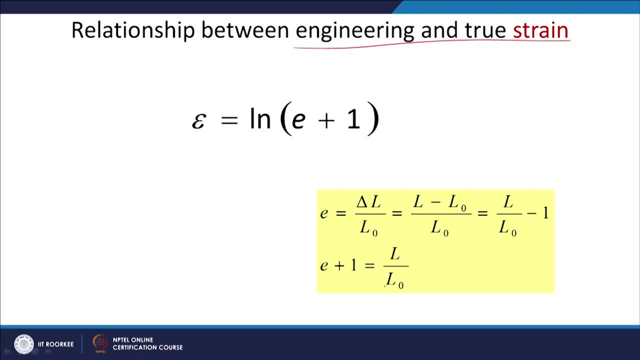 one here, So it will become E plus 1, equal to L by L0.. Okay, Now we know that what is epsilon? the true strain is lon of final length divided by the initial length. Okay, So which will look like this, so I can replace it here. so now my engineering. this is the. 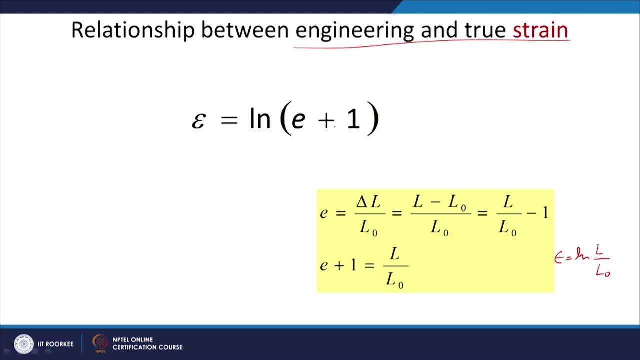 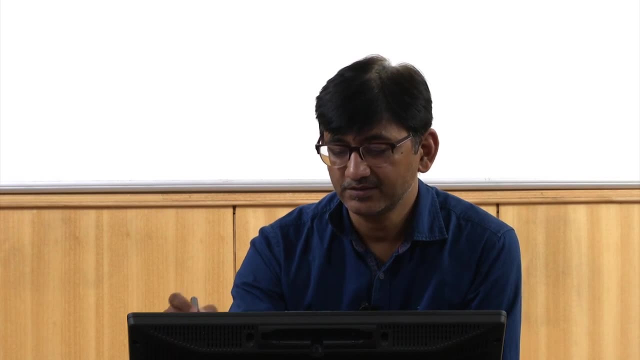 true strain. Okay, So this is basically logarithmic of E plus 1.. So whatever you calculation you do in engineering strain, you add 1 into that and take the logarithmic of that will give you the true strain. Okay, Now relationship between engineering and true stress. 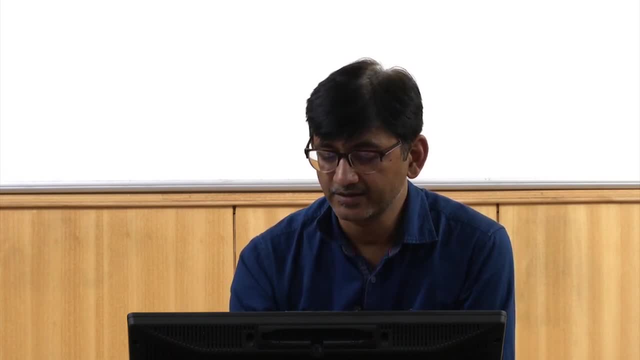 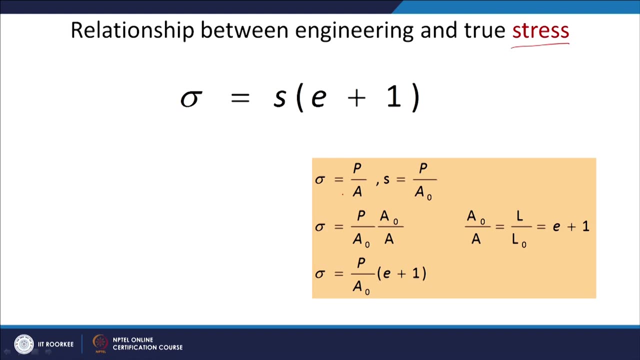 Okay, Again, let us take the in engineering stress. I will write it as P by A0. for true stress, I will write it as P by A, which is instantaneous area. Okay, So if I divide and multiply by A0 in this case, so it will become P upon A0 into A0 by. 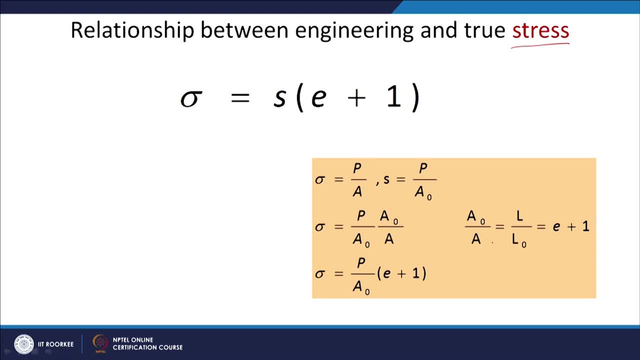 A. Okay, A0 by A can be written as L by L0.. Okay, Because, again, volume conservation, as I told you that, because in plastic deformation volume is going to be conserved. Okay, So I can write it like this: 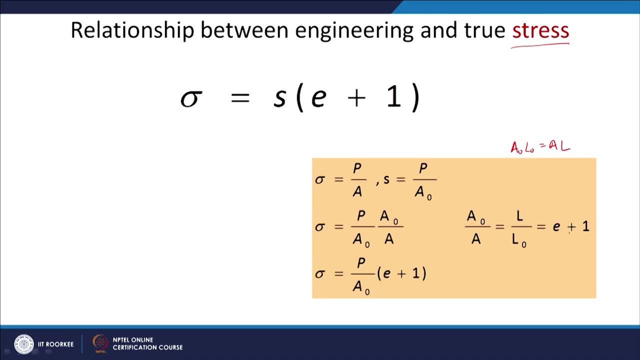 And we already know that L by L0 is equal to E plus 1. Which we did earlier in the for engineering strain calculation- sorry, engineering and true strain calculation. So L by L0 will be equal to E plus 1.. So I will be replacing here A0 by A by E plus 1. my P by A0 is equal to the engineering. 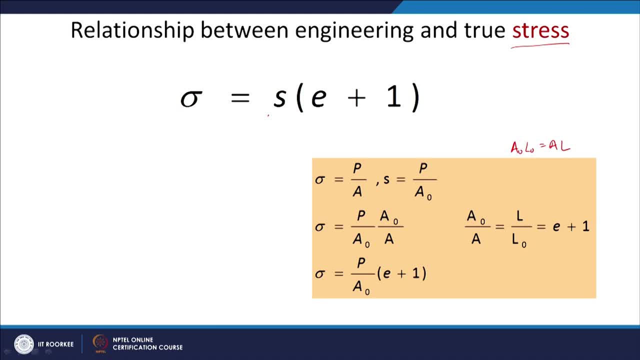 stress. Okay, So this is what I have written now: the engineering stress into E plus 1.. Okay, So this is what will be the relationship between the engineering and true stress, and the previous one is between the engineering and true strain. 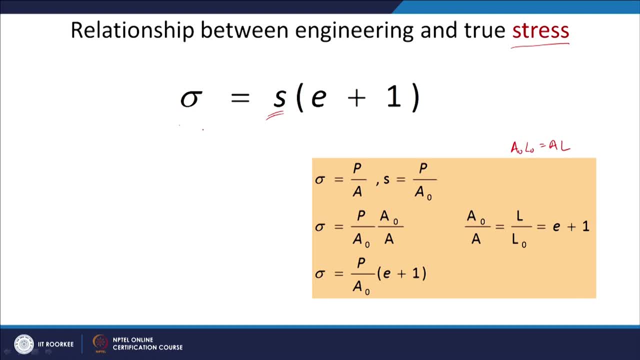 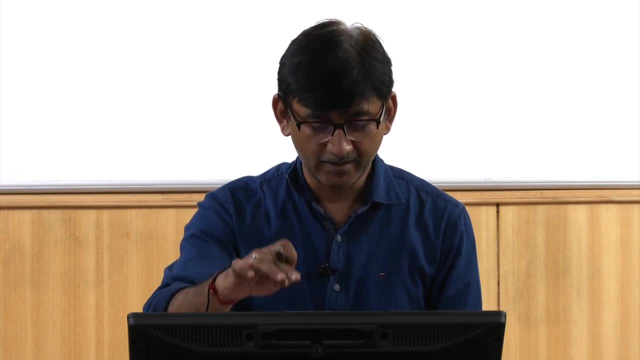 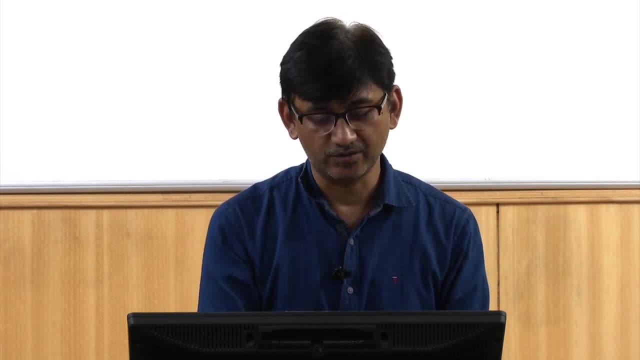 Okay, So if you know the engineering calculation also, if you have done, you can easily find out the counterpart, true stress, true strain values from that. And now let us see what will be the effect on the stress strain curve because of that. So already we have seen this red part is your. 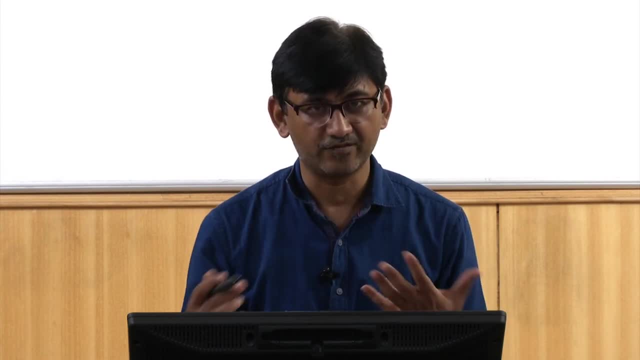 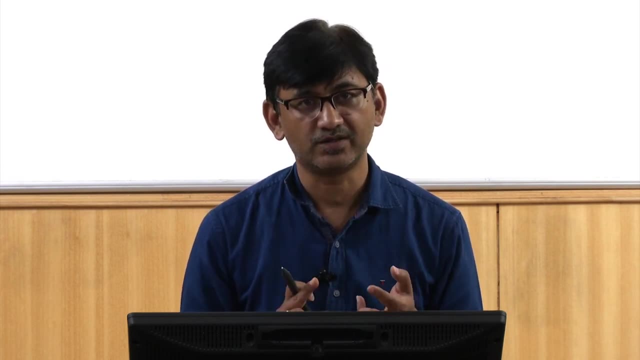 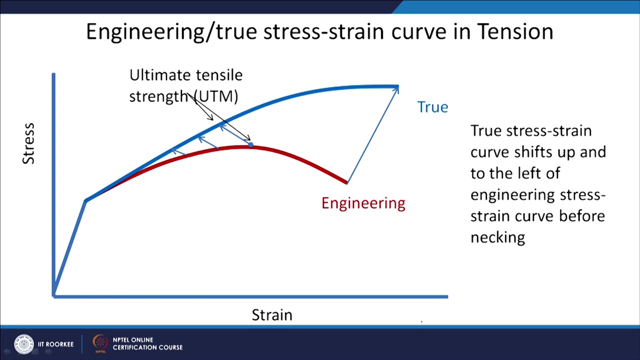 Engineering stress strain curve, which is what we have. we get from the machine. Okay, So in from machine you get the data in terms of force versus elongation, sorry, elongation versus force. So elongation will be on x axis and force will be on y axis. 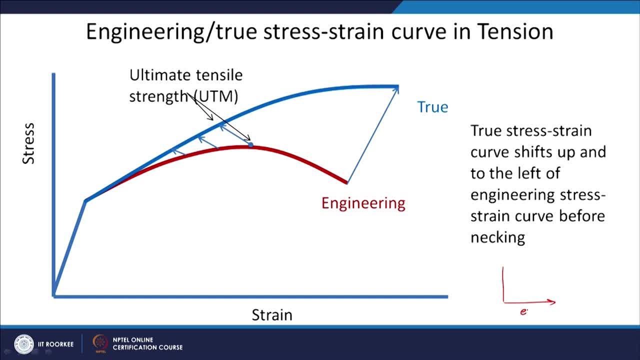 Okay, This is what I get from the machine. Okay, Elongation, and here it will be force. So elongation, If I divide by original length, then it will be equal to engineering strain Force divided by original cross sectional area. original area will give me the engineering 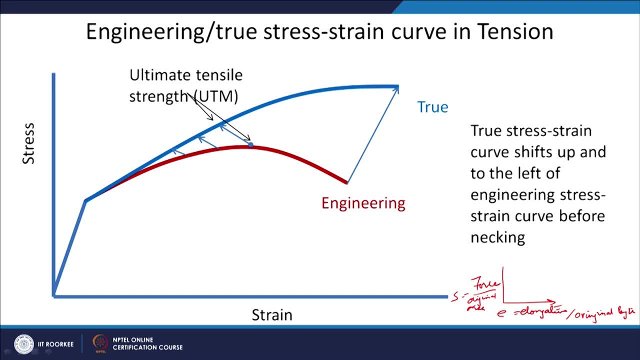 stress. So we can get that, whatever is the curve. Now, as I told you, You can find out the true stress strain curve from that. Okay, So now as I told you that when I am deforming length is increasing, 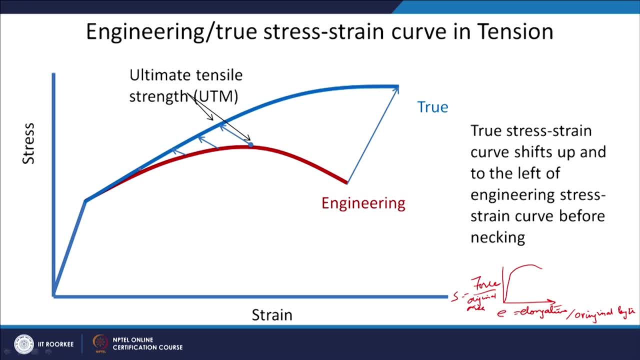 Okay. So what I am seeing is that length is increasing and area is reducing, that my stress values are more than the engineering stress. Okay, But since my length is increasing, the length, the for strain calculation it will be delta L by L. So if L is continuously increasing, that means my strain value will be lower. the true strain. 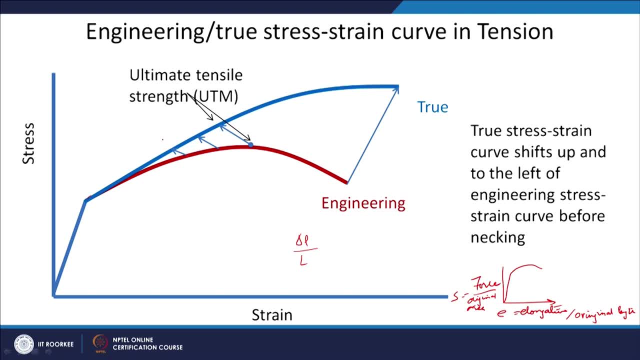 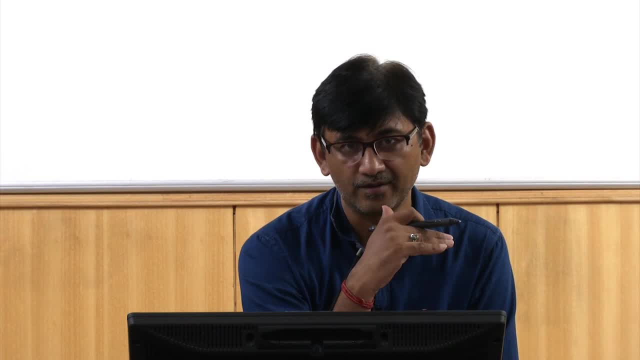 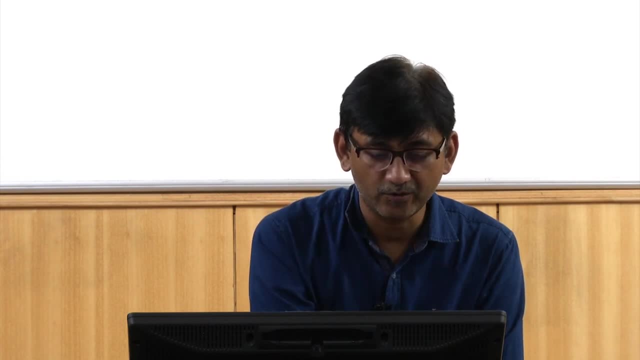 value will be lower. So you can see that the points are shown by back arrows here. So stress is going up, but strain is coming down or is showing lower value than the engineering strain, So engineering strain will be more Okay. 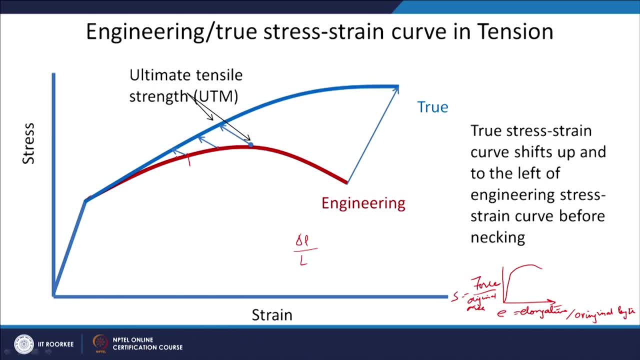 True strain for the corresponding elongation will be less than the engineering strain, So engineering strain will be more Okay, So the elongation will be less Okay, But engineering stress will be low and true stress will be high for the same amount of. 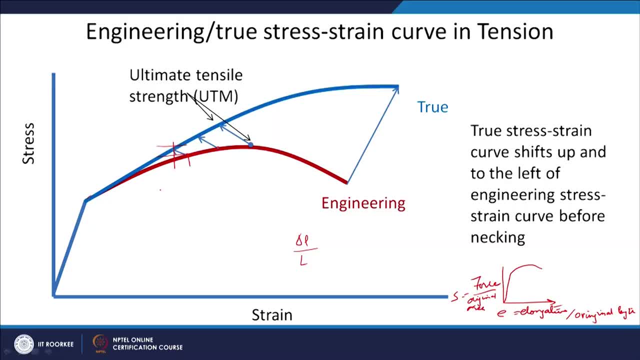 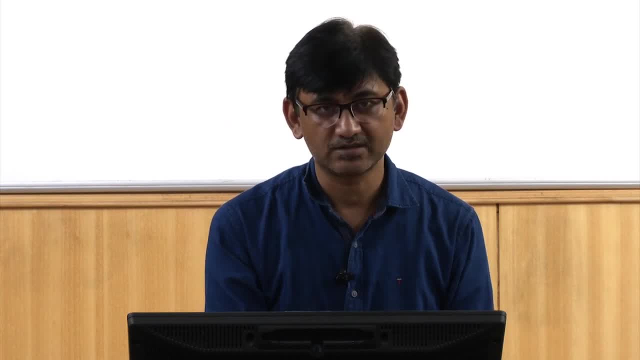 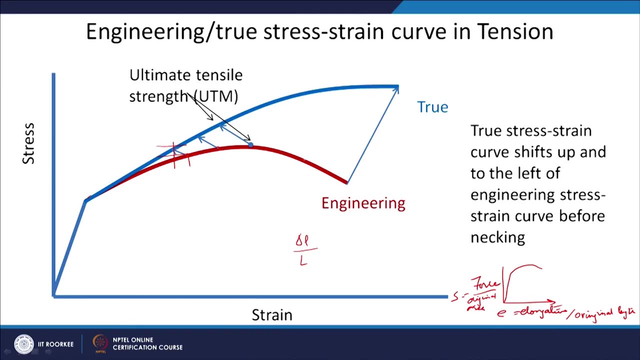 deformation. Okay, So my curve goes like in the in the: in the this side, but upward side. So this is how the true stress stress values, or the true stress stress curve, will be there and this is how the engineering stress strain curve will be there. 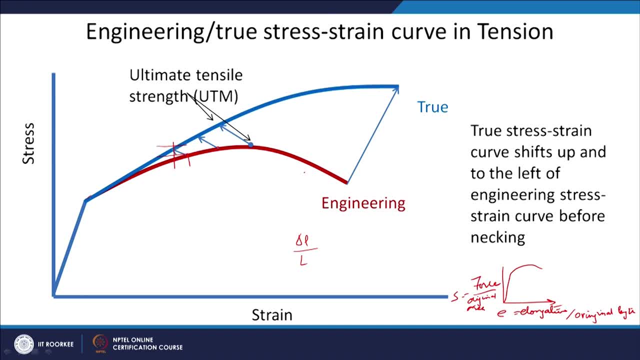 After making actually the situation become just opposite. now you can see that my the strain value is more the true strain value is more than the engineering strain. Okay, And similarly my of course stress value will always be high compared to the true stress value will always be higher compared to the engineering stress. 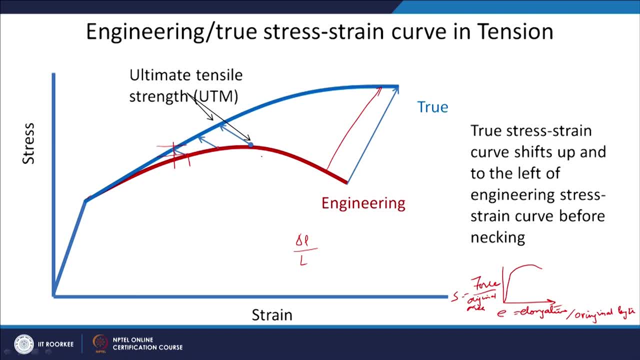 Okay. So after making, After making, basically, one thing to note is that we will take only the area and the length in the necked region, Okay, Not the overall gauge length, Okay To for the calculation of true value, Okay, 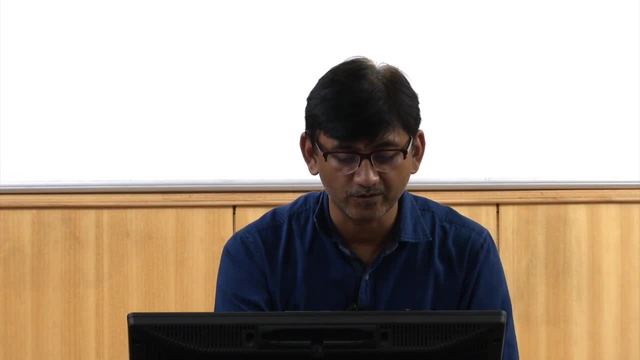 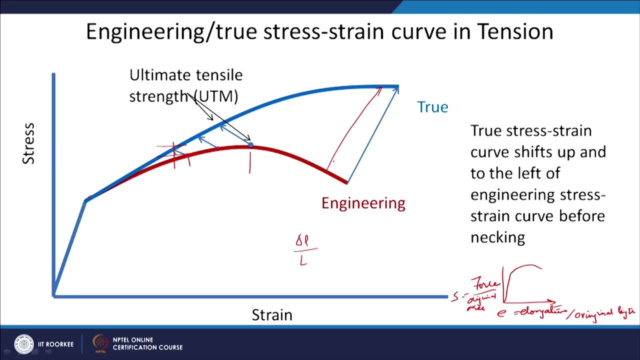 So that you have to consider that up to making. as I told you, you have a uniform elongation So I can take the whole gauge length and the cross sectional area to find out the true stress strain values and so on. But after making it will be non-uniform deformation. 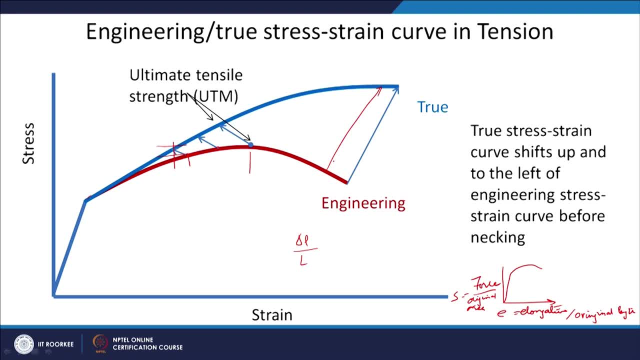 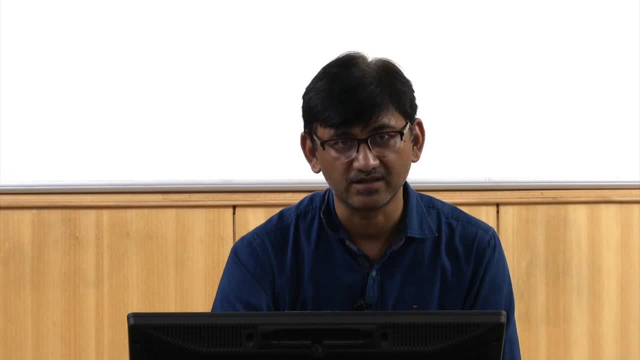 So you will take the area of the neck region and also the length where the making is taking place, and that is why you can see that my now true strain values are more than the engineering strain values. Okay, Because my length has reduced quite a lot. 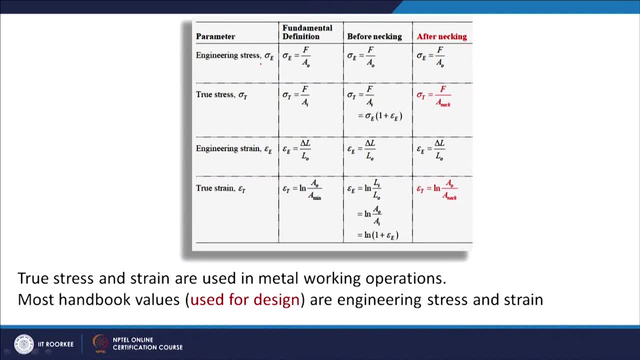 Now these are some relationships, Okay, Just to clarify to you. Okay, For engineering stress: at every point my I will be having cross sectional area as a non-uniform And force is whatever my machine is going to provide me In true stress. I am going to take force, what my machine is going to provide me and the 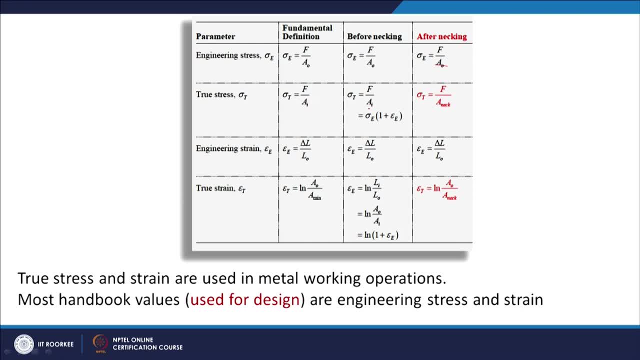 cross sectional area will be the instantaneous cross sectional area which can be given by this Up to before making. you will have this After making. as I told you, you have to take the area of the necked region- Engineering stress in case of engineering strain. 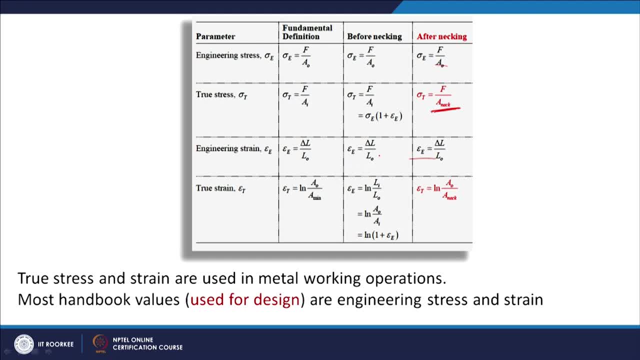 All the everywhere, you will be dividing only by L0.. In case of true strain, you will be dividing it by the instantaneous length or area. Okay, In terms of area, you can write it like this, And in terms of length, it will be L upon L0.. 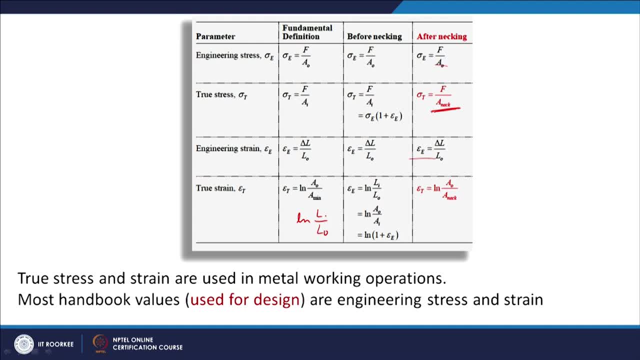 So it is just opposite. Okay, Inverse relationship is there. So epsilon E is equal to Li by L0, or A0 by Ai, and this is equal to this already. you have seen this. But in case of after necking, as I told you, you have to take the area of the neck. 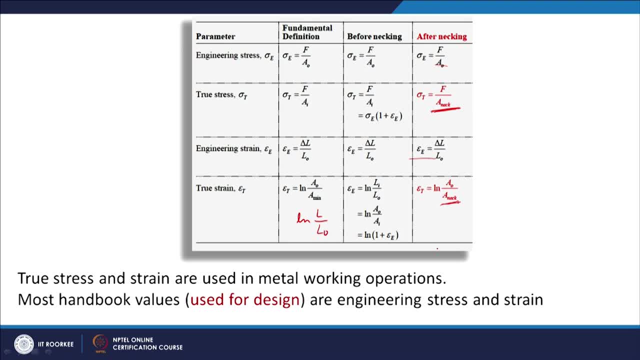 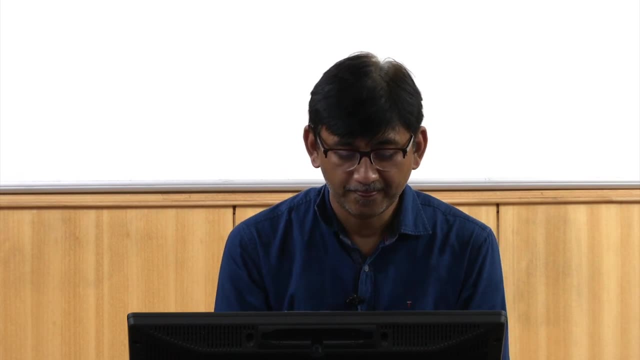 Now, as I already told you that true stress and true strain values are used in metal working operation, Okay, Because there I will do- or deform the material in stages. I cannot deform material in 1 step, Okay. But for design purposes For a material, 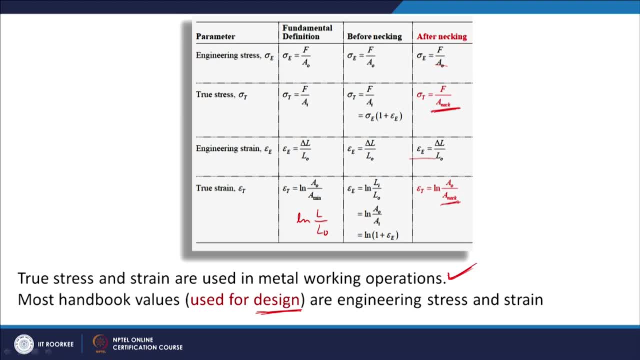 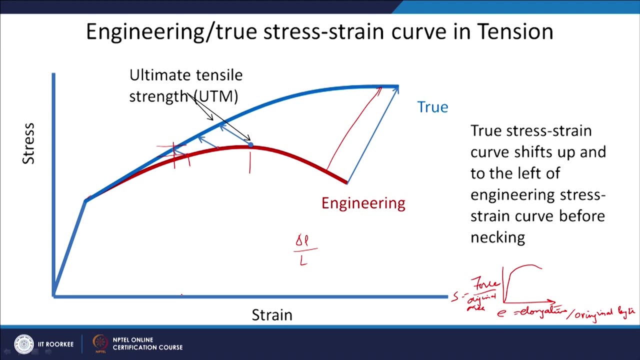 For a mechanical lequel on способabelly Okay lining structure. they need only the engineering stress and strain. they do not need true stress and strain and most of the handbook also gives only the engineering stress and strain Why we will not use the true stress strain curve. if you see here in the initial elastic 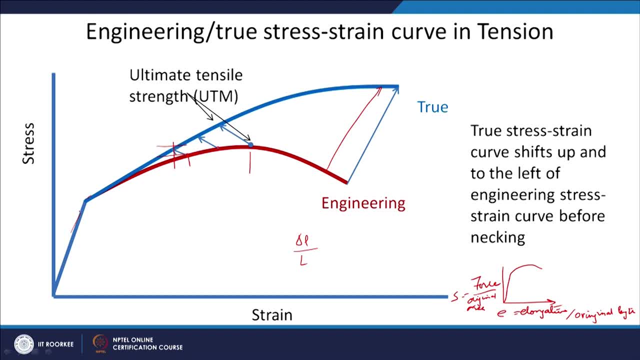 part. my engineering and the true stress strain curve are overlapping each other. there is no difference, they are same. there is not going to be any change in the value between the true and the engineering up to elastic limit and for a design engineer he will be. 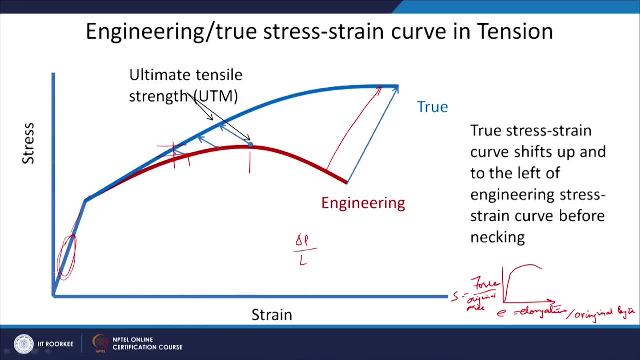 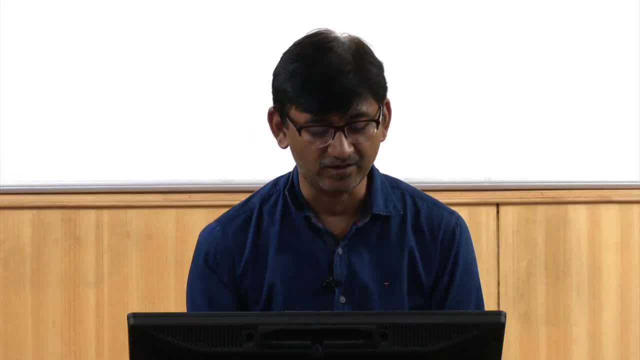 only designing the material in this range. okay, So for them, it is of no use to know the true stress and strain value. they only are concerned with the engineering stress and strain values, and this is what most of the handbooks are going to report. okay, 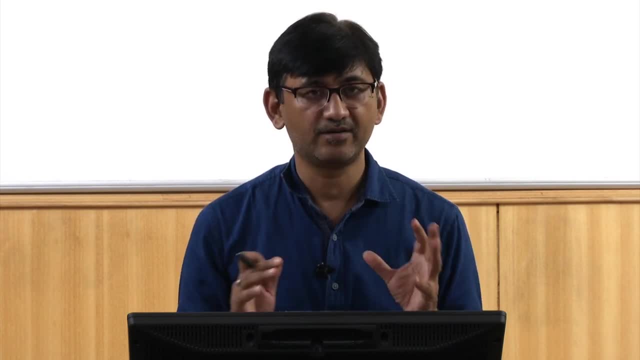 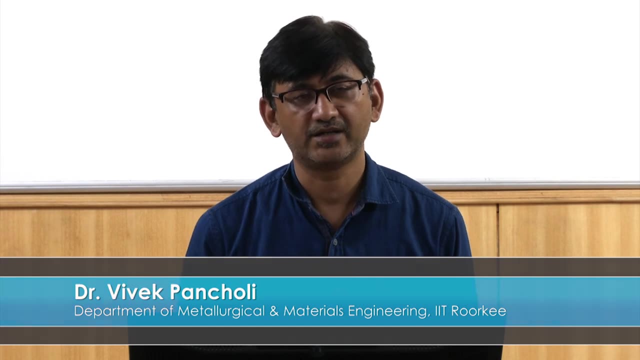 So with that I want to thank you. this is a very important lecture to understand the difference between these two parameters, So I hope you might have appreciated that why we want to do a calculation of true stress and strain. Thank you.